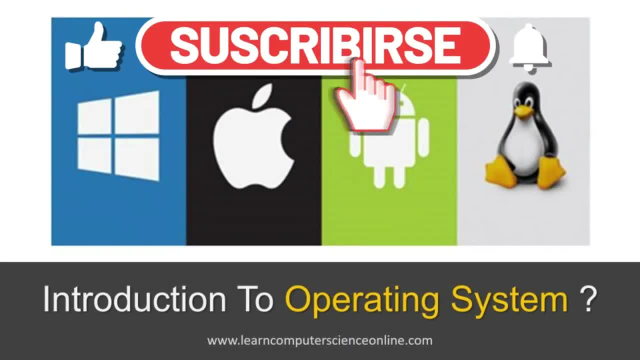 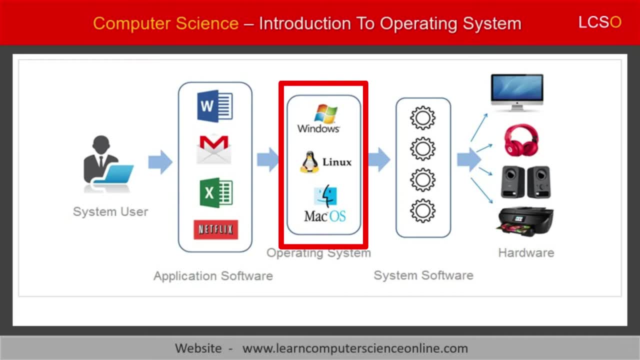 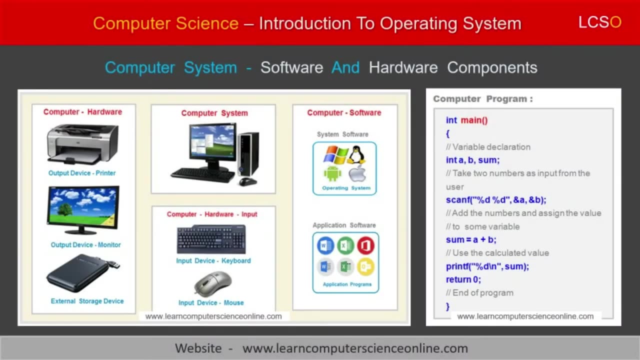 operating system. Alright, after this brief introduction, let us now dive a bit deeper to understand what is an operating system and its importance in computer architecture and organization. Let us now discuss in detail what is an operating system In computer architecture, the computer. 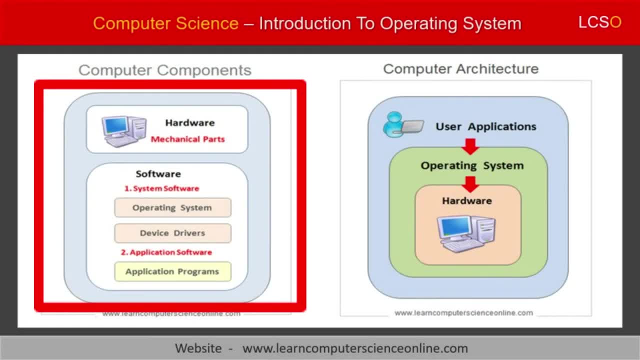 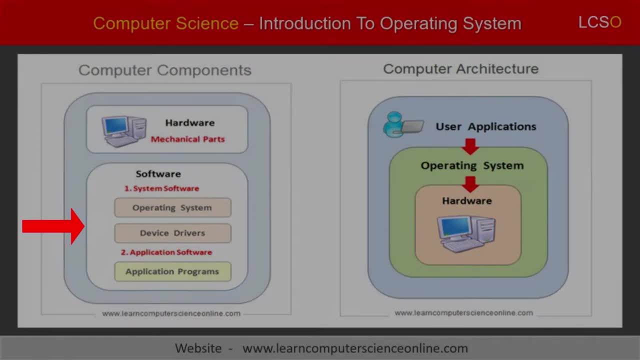 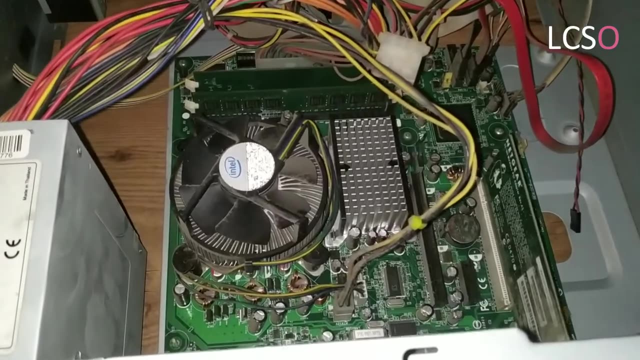 system basically consists of two types of components. These components are, First, the hardware components And second, the software components. The computer hardware is a general term used to describe the various physical components that are essential part of the 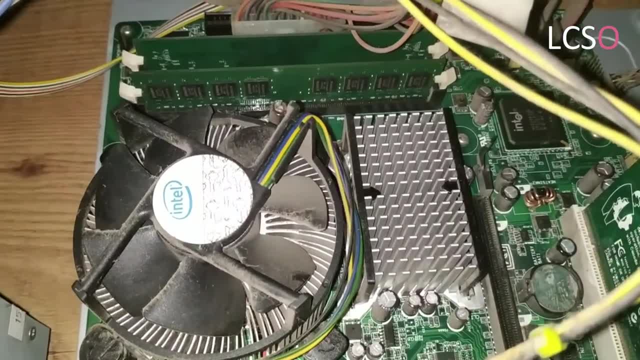 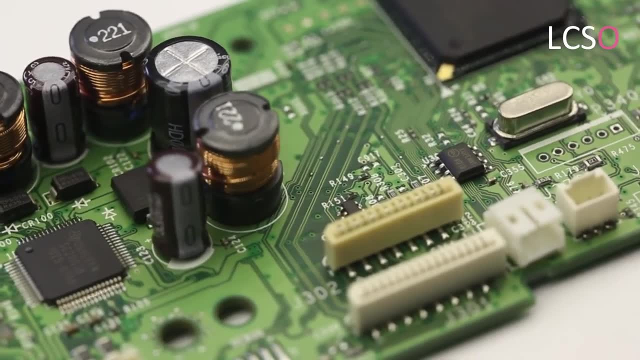 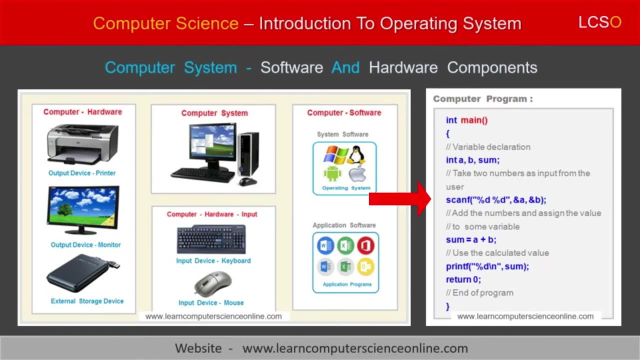 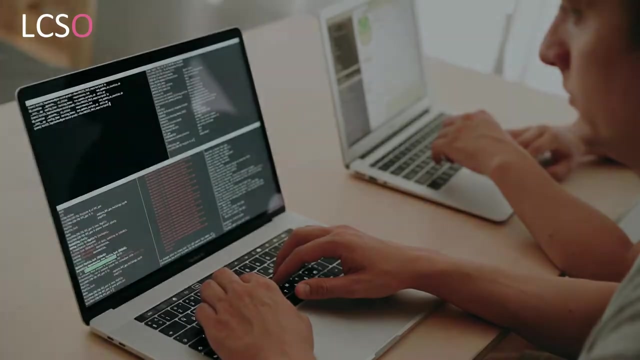 every computer system. The computer hardware includes various mechanical, electrical and electronics components used to build the computer system, Whereas the software components provide a set of instructions which directs the computer to perform a specific task. In other words, a software is a computer program used to communicate with computer. 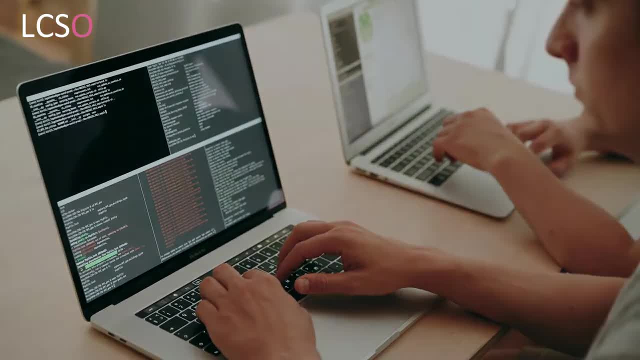 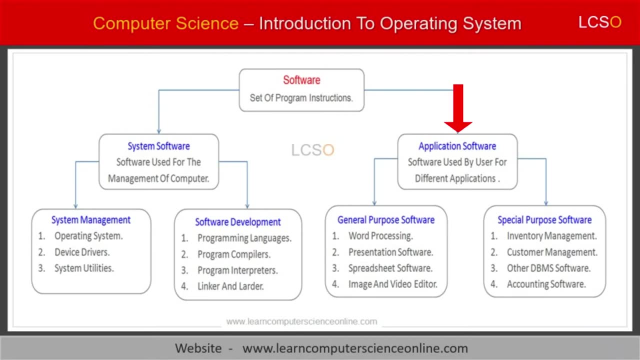 regarding the operation that we want computer to perform. The computer system needs basically two types of software components. The first type of software is the computer hardware. The computer software is called an application software, And the second type of software is called a system. 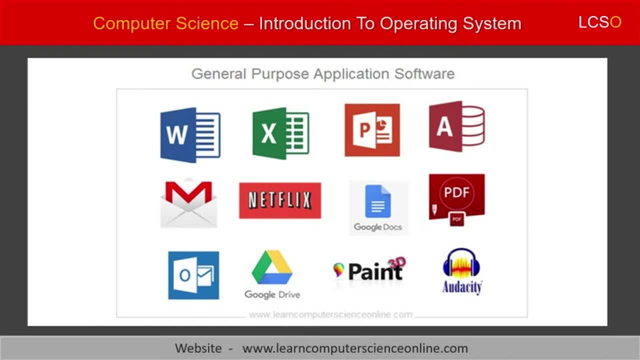 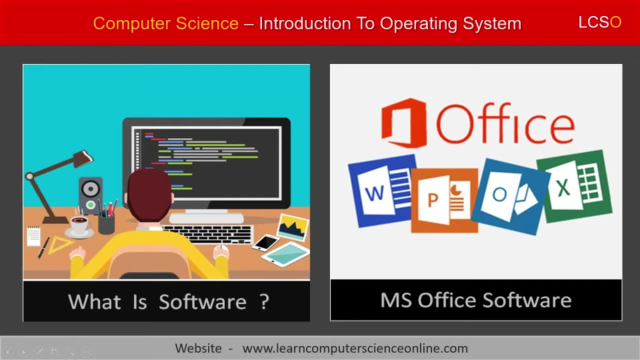 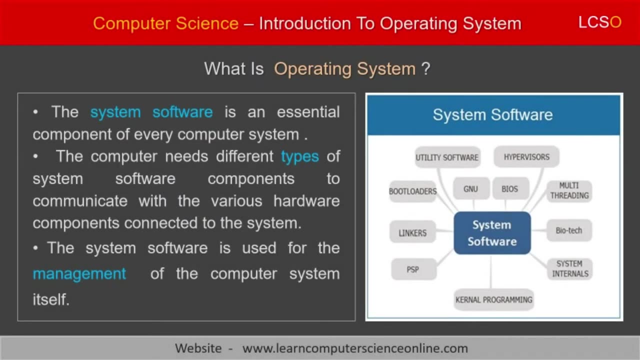 software. An application software is designed to allow the computer user to perform various tasks on the computer. For example, Microsoft Word is the most commonly used application software for creating the text documents, Whereas the system software is a special type of software internally. 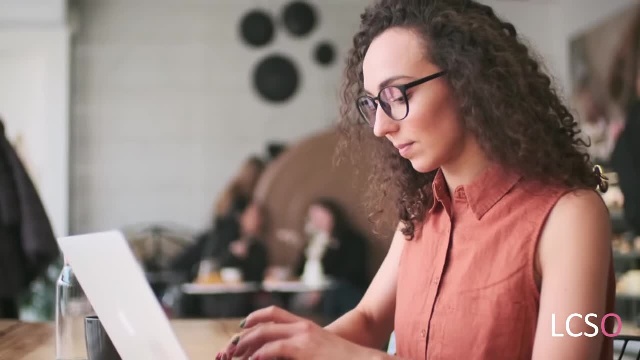 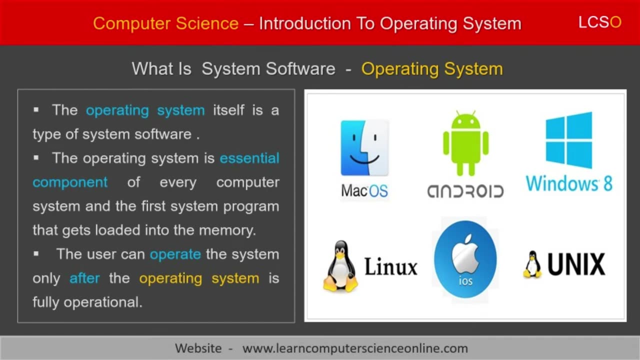 used by the computer system itself to manage an operation. The computer software is designed to operate the computer system. An operating system is the most important system software and it is an essential component of every computer When we power on and start the computer. 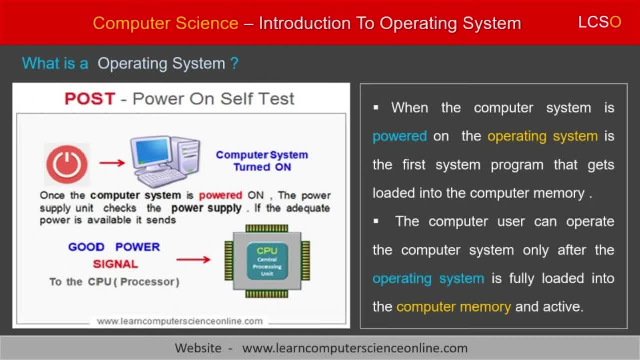 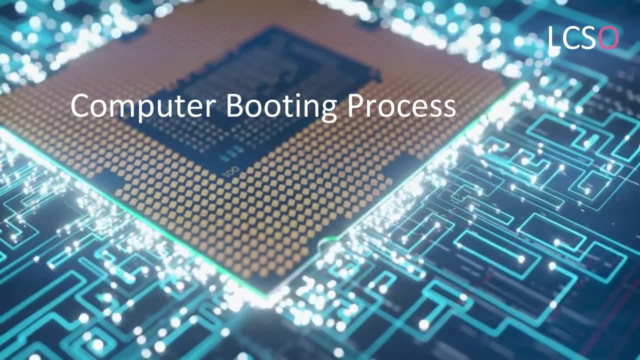 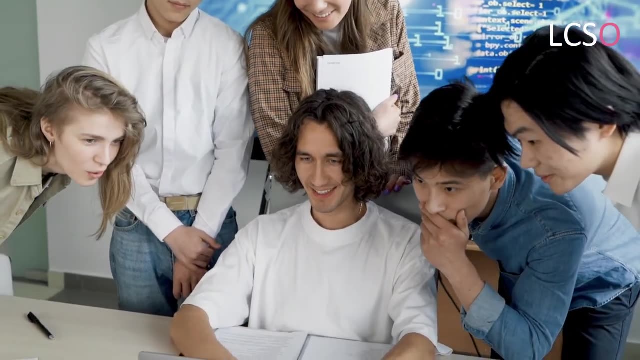 it is the operating system that gets loaded into the main memory RAM of the computer. This startup operation, which loads the operating system into the memory, is called as computer booting process. The computer user can operate the computer system only after the operating. 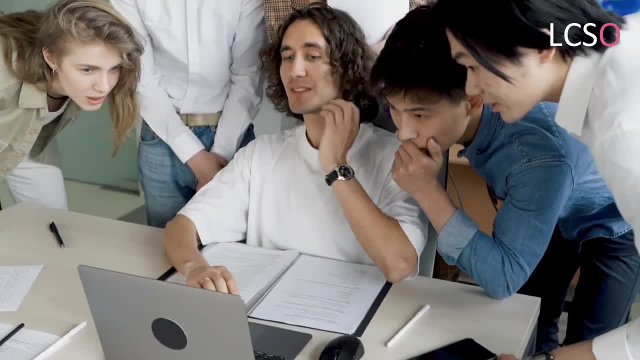 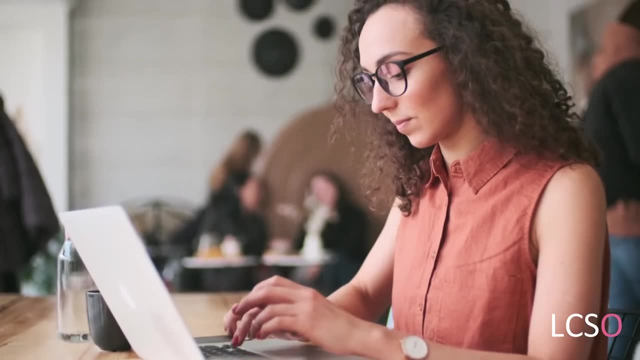 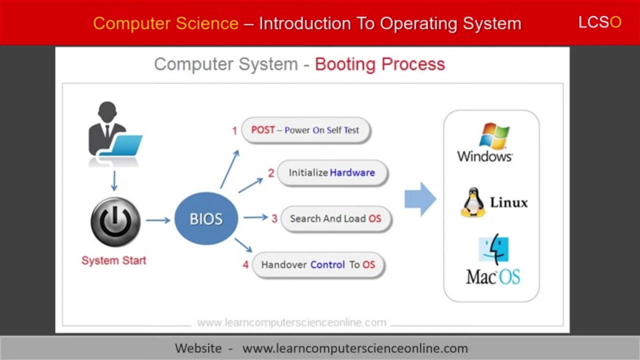 software is fully loaded into the computer memory and it is fully operational. Once the operating system is fully operational, the computer can be used by the user to perform various tasks on the computer. The computer system booting process is managed by a special program called. 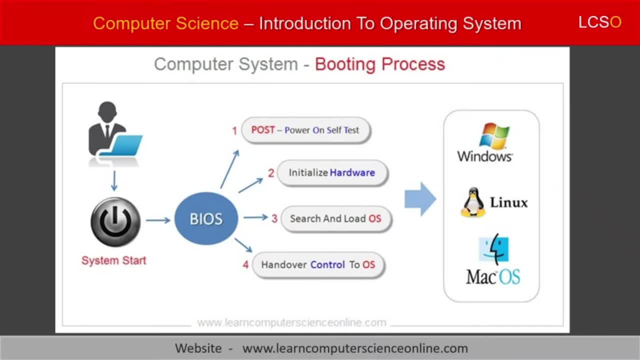 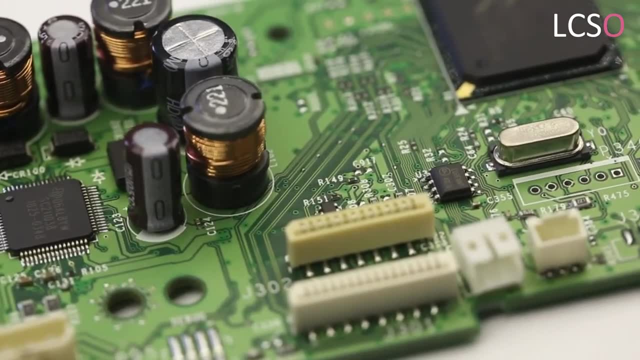 the BIOS startup routine. The term BIOS stands for basic input output system. The BIOS program is a type of firmware that resides into the BIOS chip Based on the computer motherboard. The main function of the BIOS software is to load the 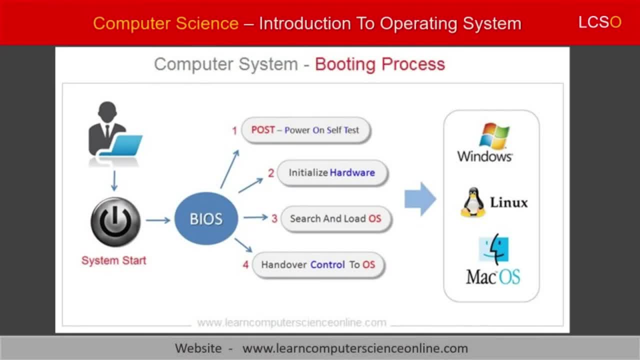 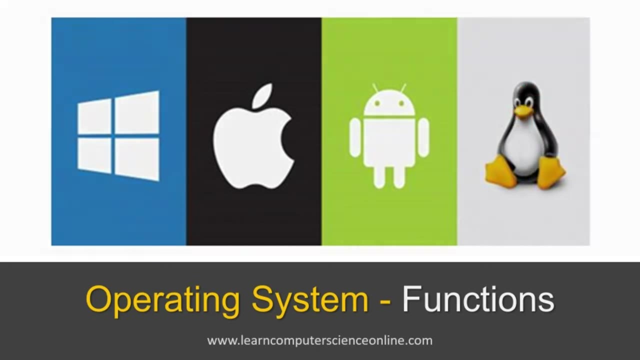 operating system, And therefore the BIOS, comes into action each time we switch on the computer. The operating system gets the control of the system after the booting process is complete. Let now briefly discuss some important functions performed by the operating system. 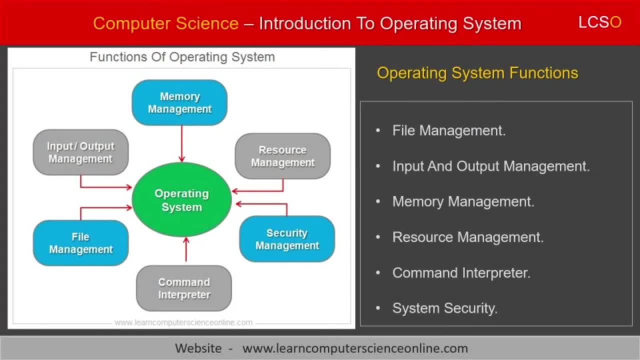 As discussed earlier, the operating system performs several important functions. The operating system performs several important functions. The operating system functions include file management, process management, resource management, memory management, command interpreter and the system security. Let us now discuss some important features of the operating system. 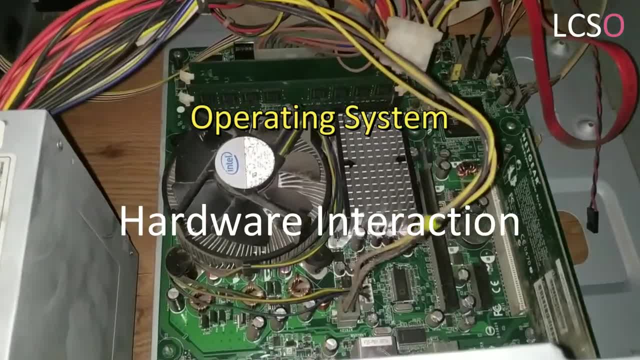 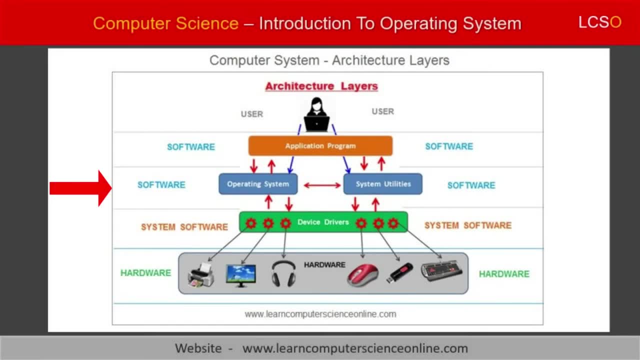 The hardware interaction is the most important feature of the operating system. Let us discuss this topic in detail. In computer architecture, the operating system works as an interface between the application software and the computer hardware. The application software is designed to allow the computer user. 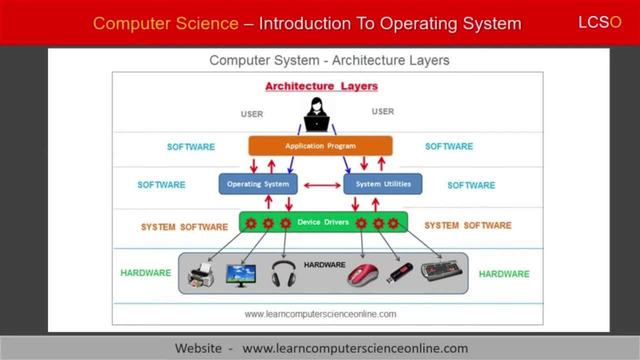 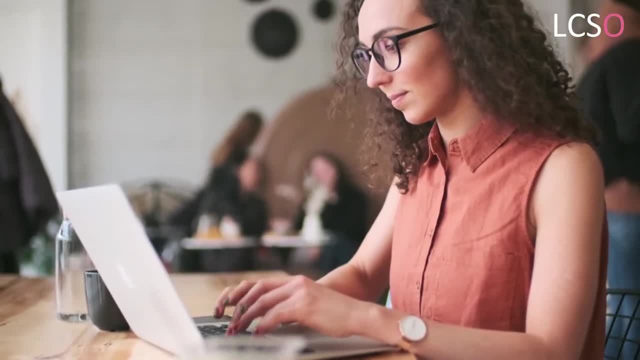 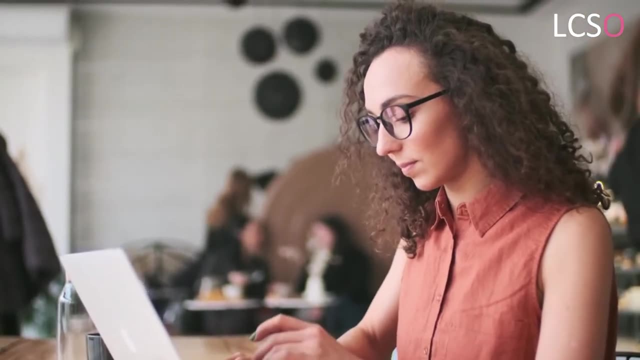 to perform various operations on the computer. These operations might also include some hardware interaction. For example, a computer user might use the Microsoft Word program to create a text document. In some cases, the user might also want to use the printer. 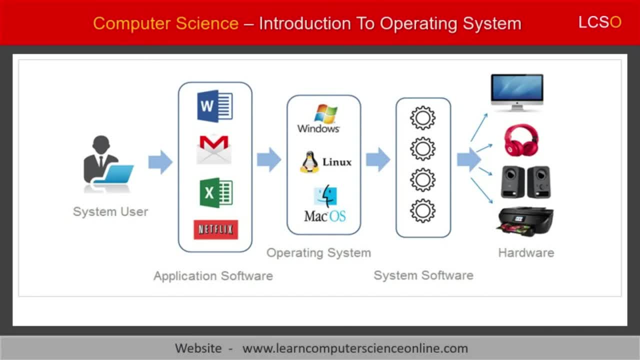 connected to the system for taking the printout of the document. However, the application program used by the user cannot directly communicate with the computer hardware And therefore, in order to communicate with hardware, the application program needs operating system. 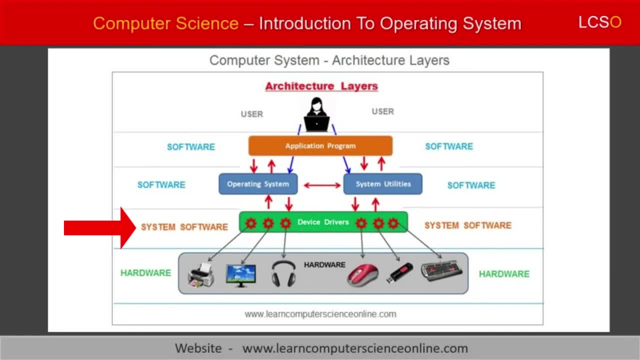 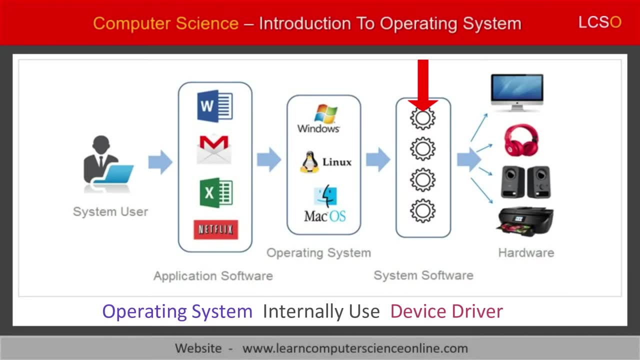 to communicate with the hardware device, The operating system internally makes use of another piece of system software called the device driver. It is the device driver software that internally communicates with various hardware components to execute various operations to be